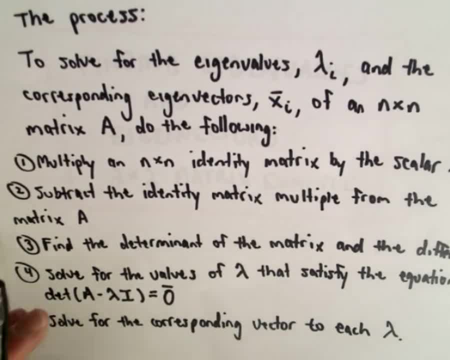 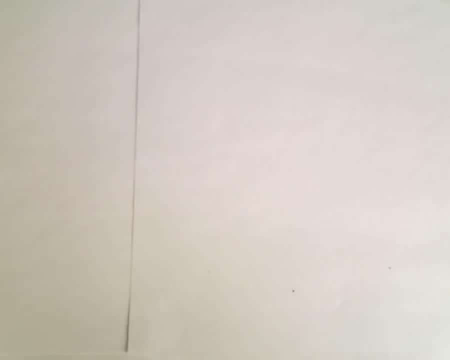 And then we're going to solve for the corresponding vector to each lambda. So let's do that here. So a few steps, but you should be able to hopefully go through it relatively quickly. So just to write everything down. Okay, so we're going to find the eigenvalues and eigenvectors of the matrix A, with entries 7,, 3, 3, negative 1.. 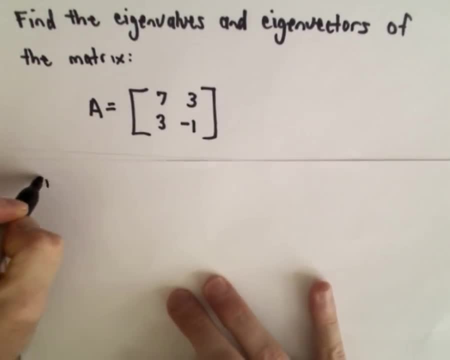 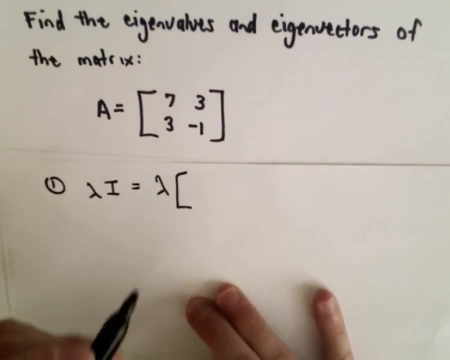 Okay, so the first step again. you know we'll just take lambda and multiply that by the identity matrix, So that's just going to be lambda Again. the identity matrix for a 2 by 2 matrix will have entries 1, 0,, 0, 1.. 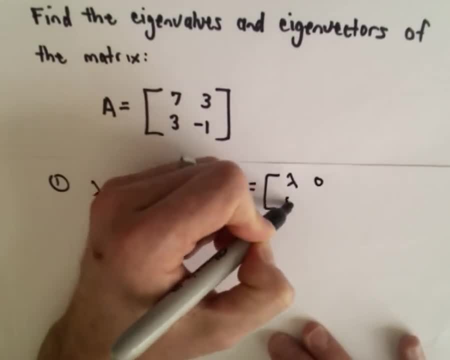 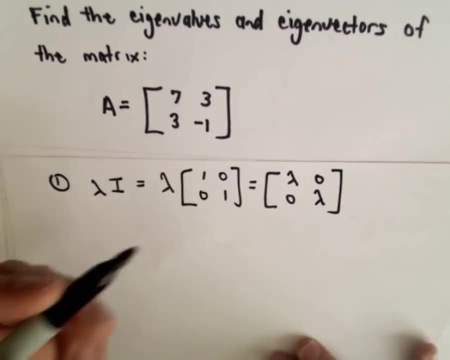 So that just gives us lambda, 0,, 0, and lambda. So again, you'll just have lambdas along the diagonal of your identity matrix. Well, it will no longer be an identity matrix, but you'll just have lambdas along the diagonal and 0s everywhere else after you multiply the identity matrix. 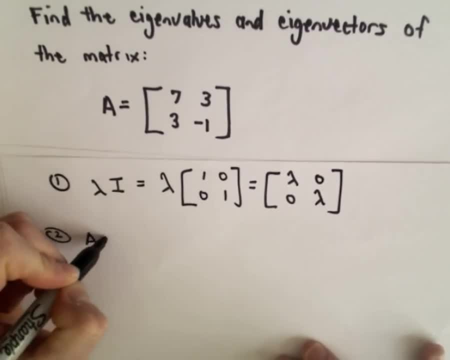 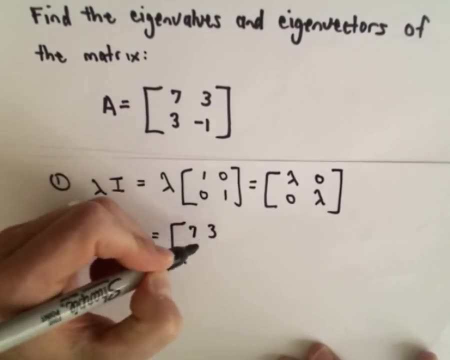 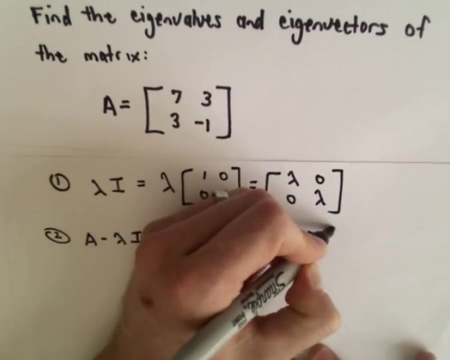 So step 2, we'll take our matrix A and subtract lambda times I. So in this case, our matrix A again has entries 7,, 3.. 3, negative, 1. And it says just subtract lambda 0,, 0, and lambda. 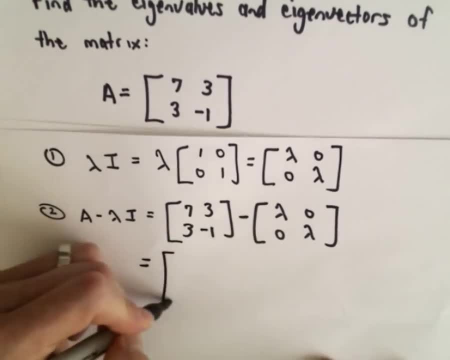 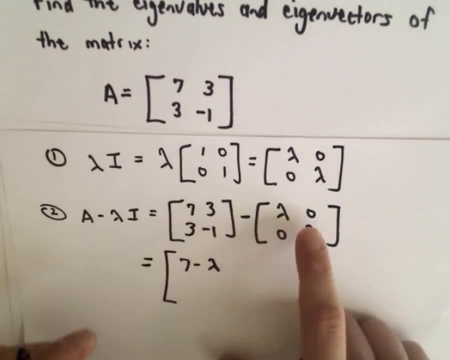 And again, remember, you just subtract respective entries. So the first, the top left entry, will be 7 minus lambda. Then we would have 3 minus 0, which is just 3.. We'll have 3 minus 0,, which again will just give us a 3.. 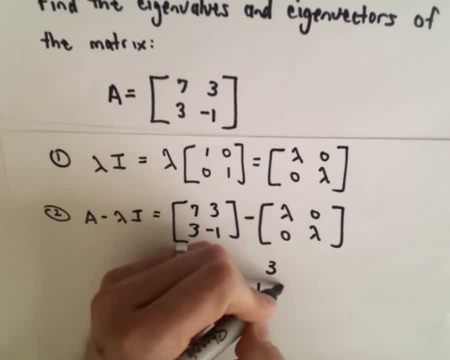 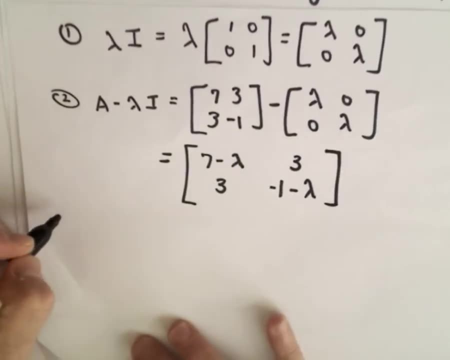 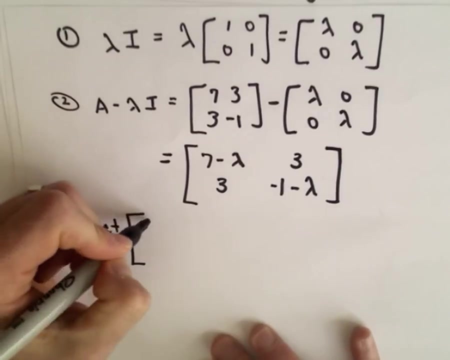 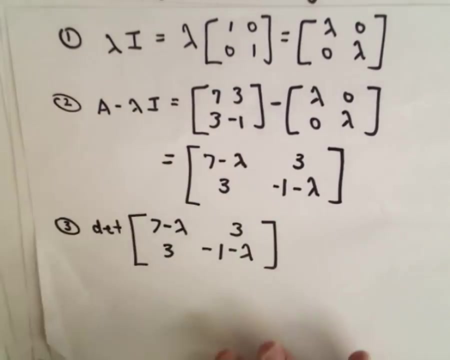 And then we'll have negative 1 minus lambda. Okay, So those are our four entries. Now step 3, the way we had it labeled a second ago- we're going to find the determinant of this matrix. So we're going to find the determinant of the matrix with entries 7 minus lambda, 3, 3, and negative 1 minus lambda. 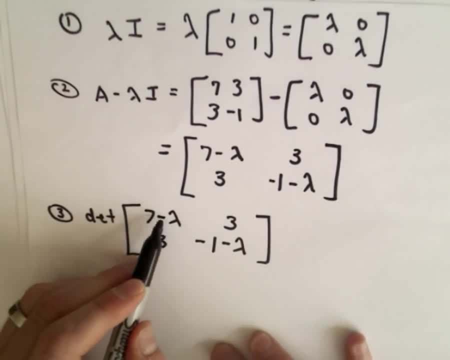 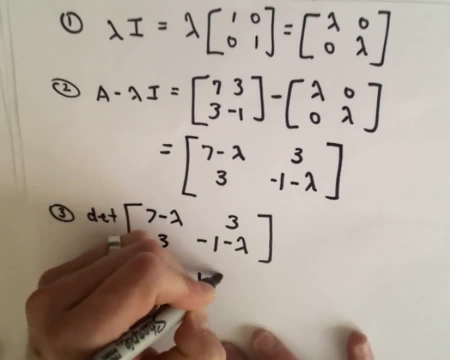 And recall. to find the determinant of a 2 by 2 matrix, we take the top left entry, multiply it by the bottom right entry, So we'll have 7 minus lambda multiplied by negative 1 minus lambda. Then we use a minus sign. 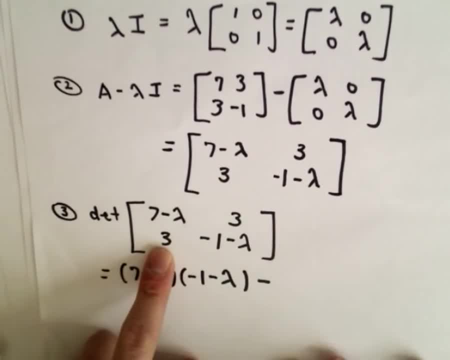 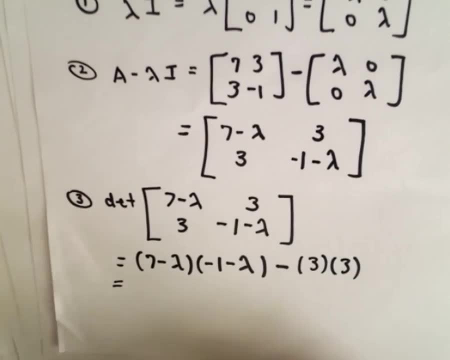 We take the bottom left entry, multiply that by the top right entry, So we'll have 3 multiplied by 3.. Okay, So let's see. if we can't simplify this, We'll have negative 7. It looks like minus 7 times lambda. 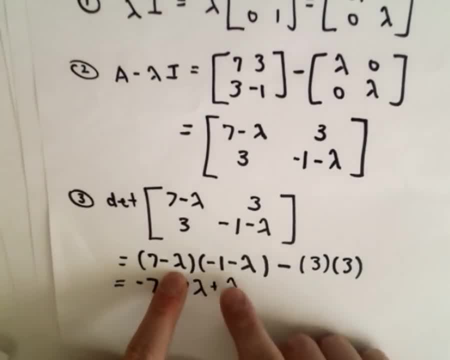 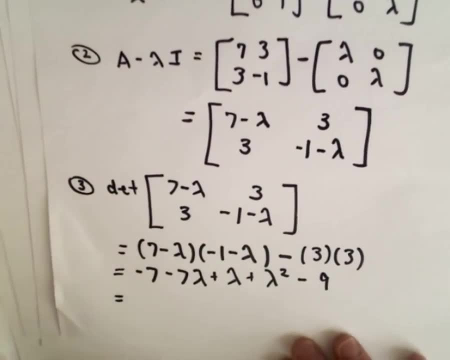 We'll have a positive lambda And then negative lambda, and negative lambda will be positive lambda squared. Then we'll have minus 9.. So I'm going to write that as lambda squared. It looks like we're going to have a negative 6 lambda. 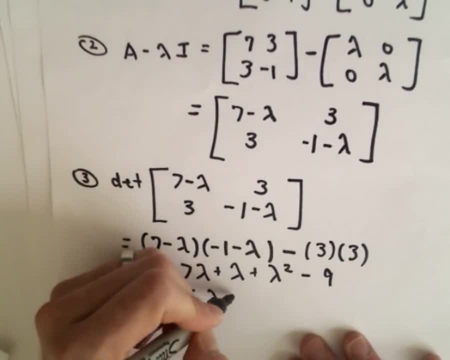 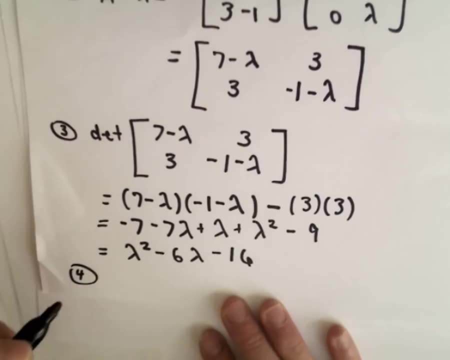 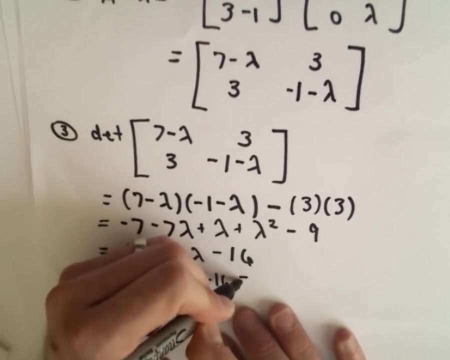 And then negative 7 minus 9.. That's going to give us just negative 16.. Okay, So step 4, I think I can put it in here. We take that equation to lambda squared minus 6, lambda minus 16.. 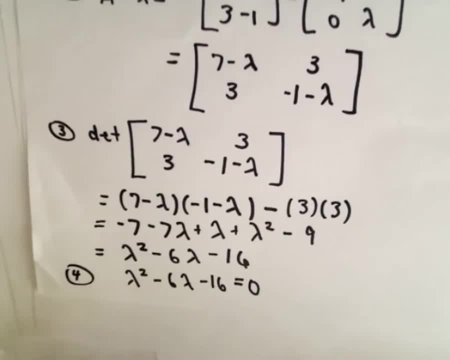 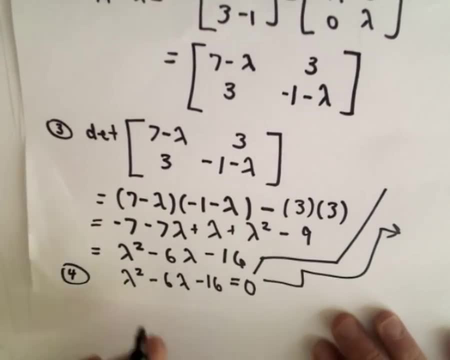 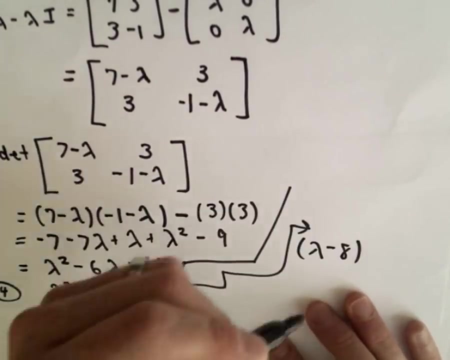 We set that equal to 0. And we solve for lambda, So no need to waste paper. So lambda squared minus 6, lambda minus 16, that's going to factor. That just factors, as I guess, lambda minus 8 multiplied by lambda plus 2.. 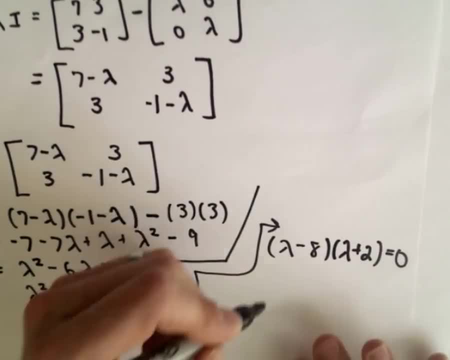 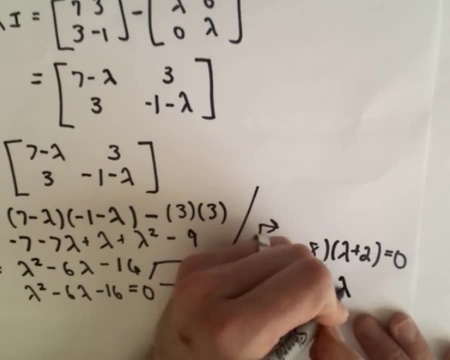 So we'll set that equal to 0.. Well, if you set each factor equal to 0, we'll get the solutions of lambda equals 8. And by setting the second factor equal to 0, we'll get lambda equals negative 2.. 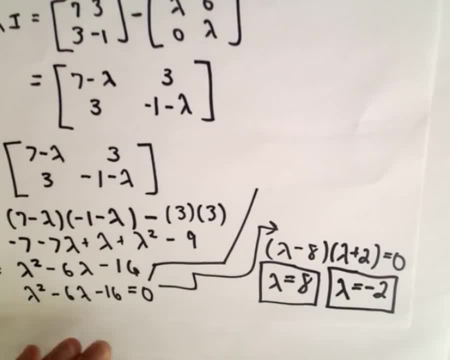 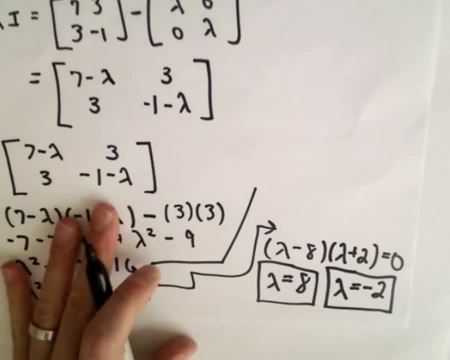 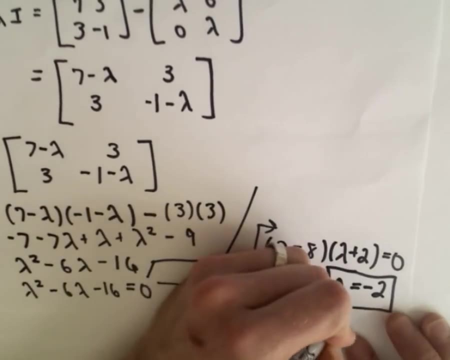 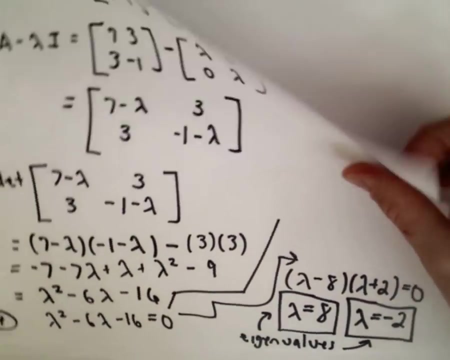 Okay, So now we've got our values for lambda. Those are going to be our eigenvalues. Okay, So these are the eigenvalues, And now we're going to need to find the corresponding eigenvectors. Alrighty, So what we do now? 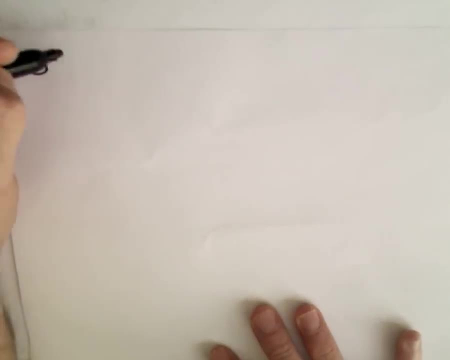 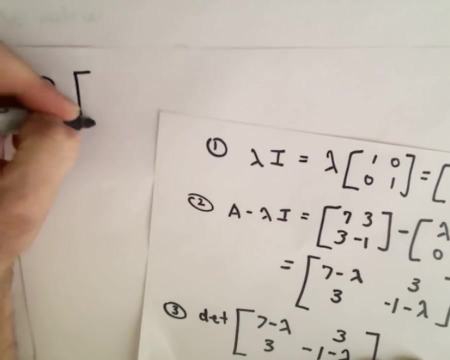 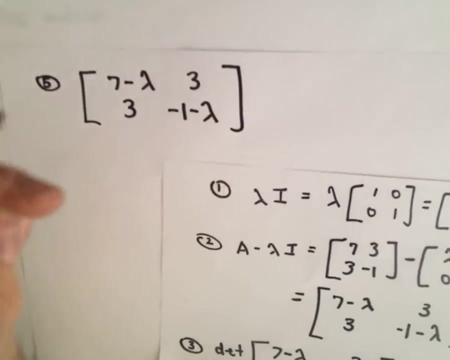 Step 5, we look at that matrix. we formed the A minus lambda I, So that was again the matrix that we found here, So I'm going to rewrite that. So we've got 7 minus lambda, 3, 3, and negative 1 minus lambda. 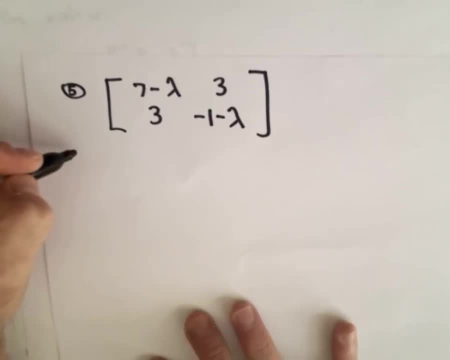 And now we've got to do a few more computations. Okay, So the first thing I'm going to do is I'm going to start with my lambda value of positive 8.. We substitute that in, So we'll get 7 minus 8.. 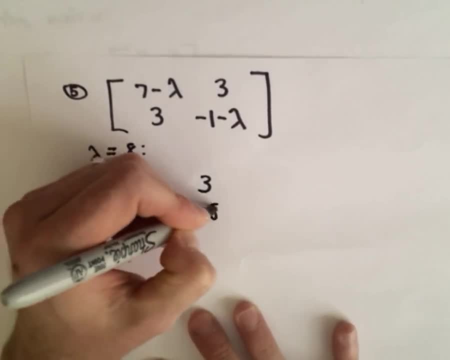 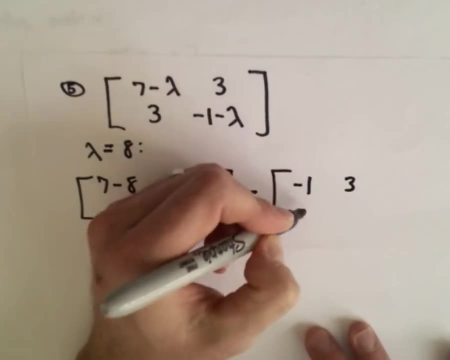 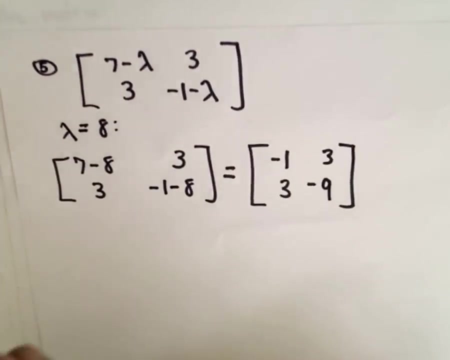 We still have a 3, a 3.. Then we'll have negative 1 minus 8. And that's going to give us negative 1,, 3, 3, and negative 9.. So now what we do. I think in my original notes maybe I called it A. 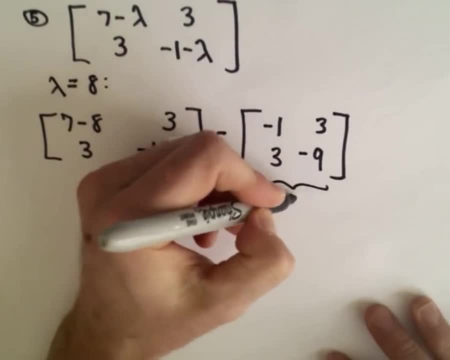 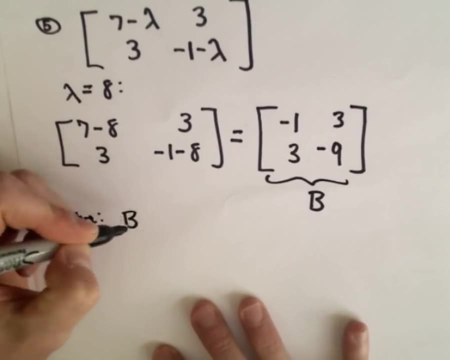 Our original matrix was A, So let me maybe call this- I don't know, I'll call this the matrix B. Now what we do is we solve the equation. We'll take matrix B multiplied by the vector x equals 0. We have to solve this. 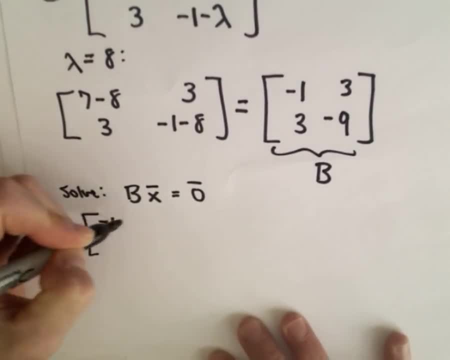 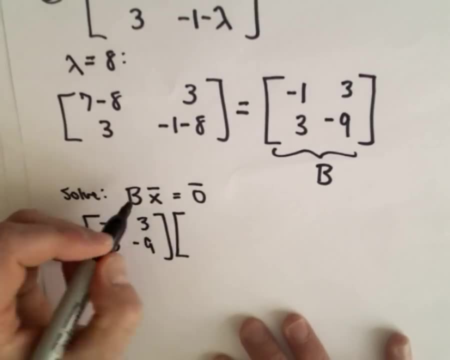 So what we want to do is we want to solve. we've got negative 1 times 3 times 3 times negative 9.. The matrix with the corresponds to the vector x. here We'll just write little x sub 1 and x sub 2.. 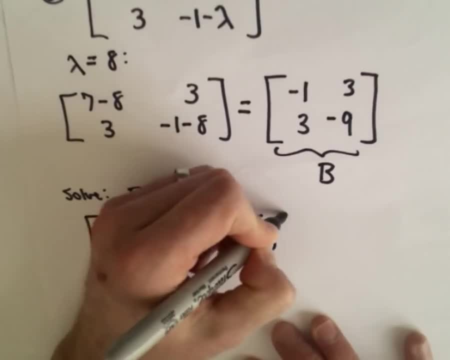 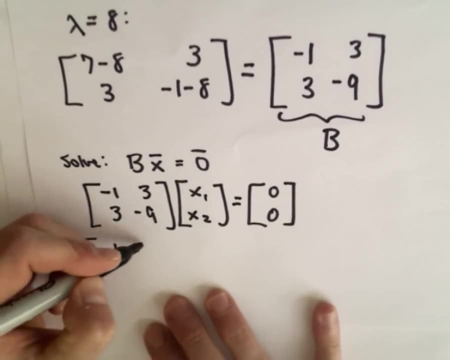 And then we've got our 0 vector here. So to solve this, I'm just going to use a little bit of row reduction So we can write this as negative 1,, 3,, 3,, negative 9.. There's my 0s. 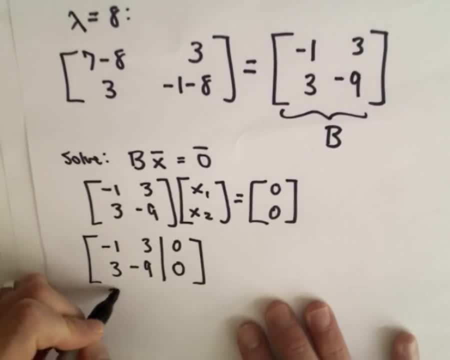 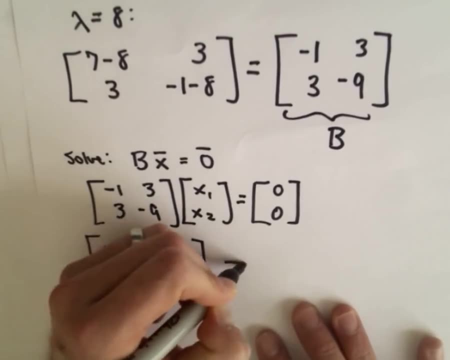 I'm just going to do some row reduction. So to solve this, it looks like to me we could take 3 times row 1, add that to row 2 to give us our new row 2.. So if we do that, the first row, nothing's going to change. 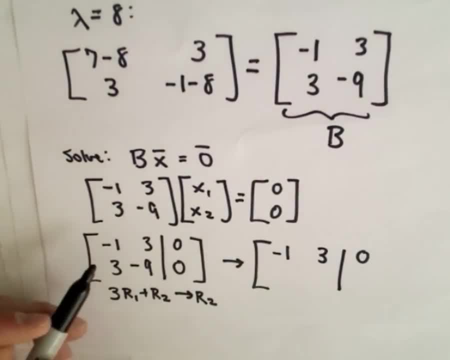 We'll have negative 1, 3, and 0. So negative 1 times 3 plus 3 will give us 0.. 3 times 3 will be 9, plus negative 9 will give us 0. And we still have a 0 at the bottom. 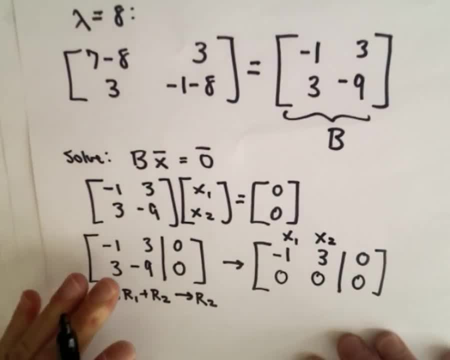 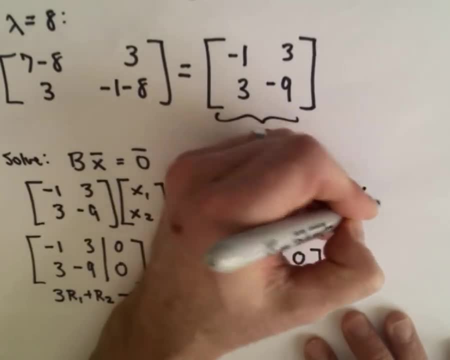 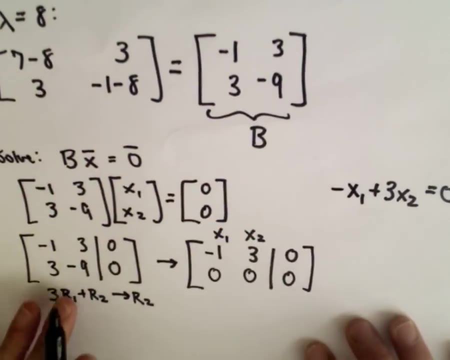 So again, this is now going to correspond to x1 and x2.. So that gives us our relationship. It says that It says that negative x1. Plus 3 times x2 equals 0. And we can simply add the x1 over and write that as 3 times x2 equals x1. 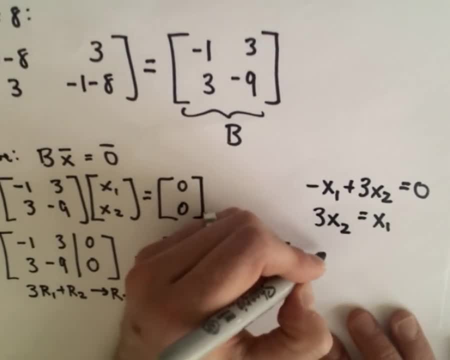 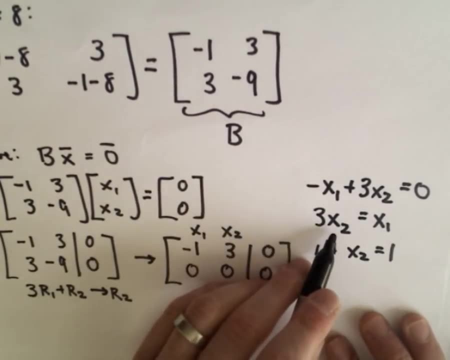 And now all you have to do is just pick some values. So the easiest ones to me, I'm going to let x2 equal 1.. And if we let x2 equal 1, well then we'll have 3 times 1.. 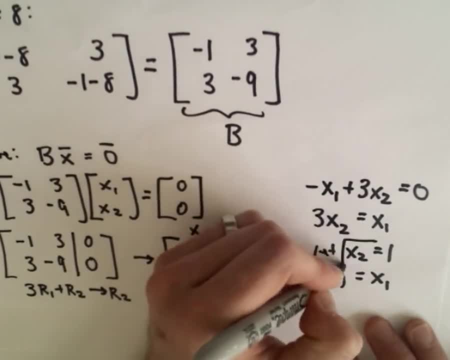 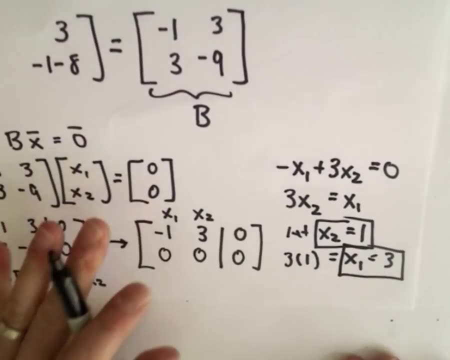 Which will give us our value for x1.. So it says, if we let x2 equal 1, it says x1 is going to equal 3.. That's going to be the eigenvector that corresponds to the eigenvalue of 8.. 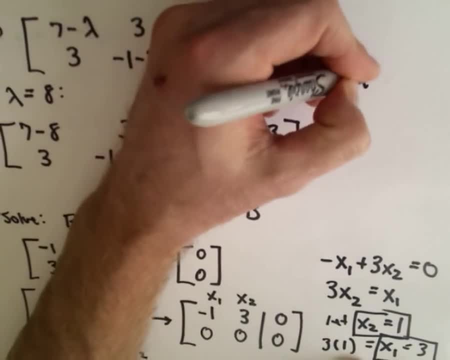 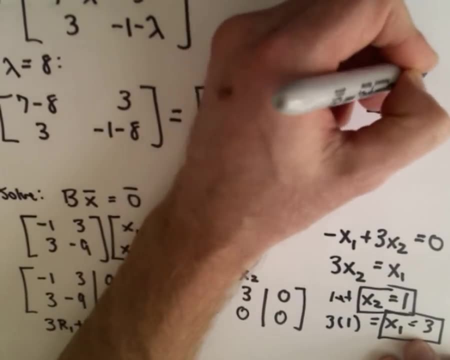 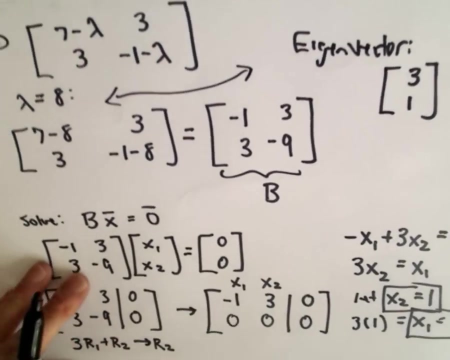 So the eigenvector? The eigenvector in this case will be the vector with entries 3 and 1.. Okay, so that eigenvector again goes with the eigenvalue of 8. And you can check, you know, if you want to. 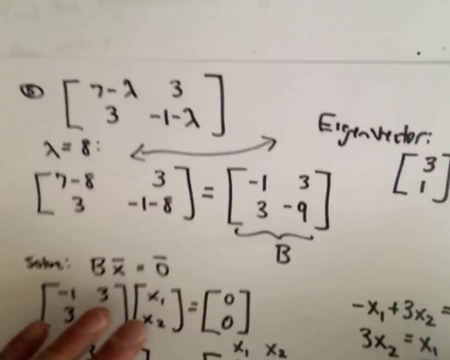 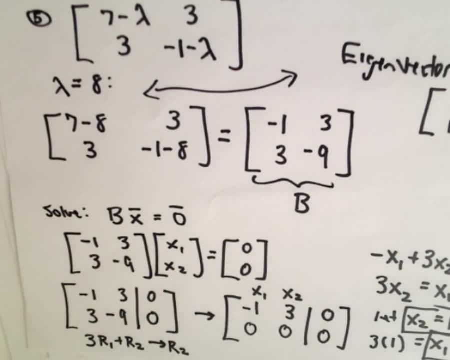 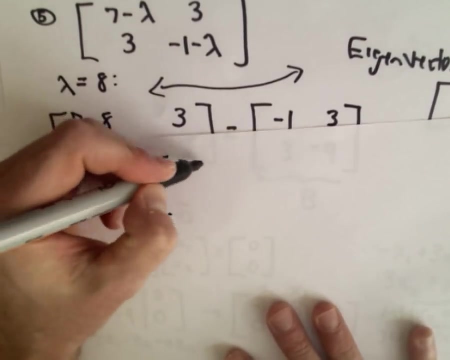 You can take the very, you know the matrix that we started with: 7,, 3,, 3, negative 1.. Let me write this down. You can check that if you take that starting matrix, 7,, 3,, 3, negative 1.. 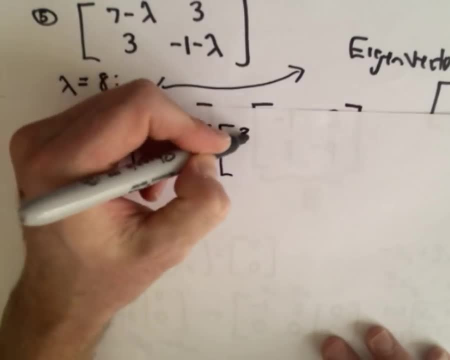 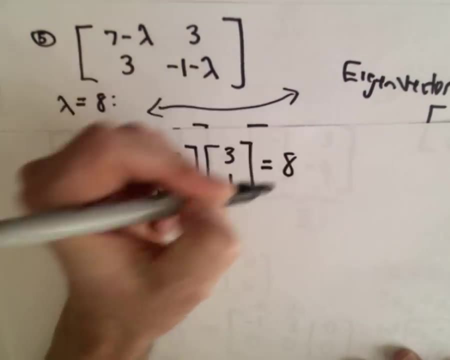 If we multiply that by our eigenvector again, which has entries 3 and 1. That'll be the same thing as when we take our eigenvalue, which is 8. And multiply that by the eigenvector of 3 and 1.. 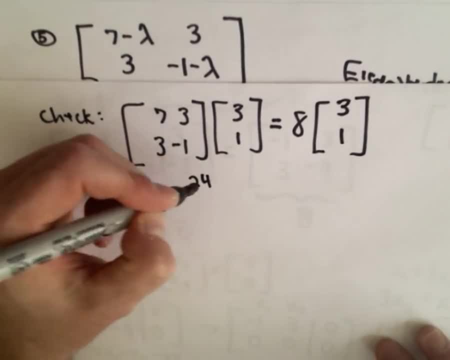 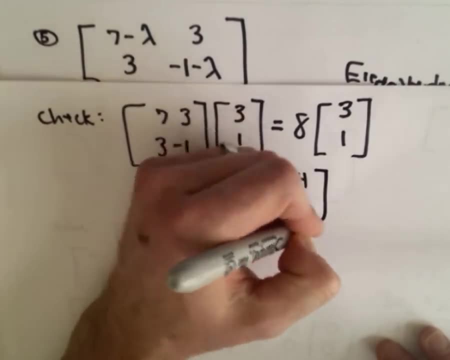 You can check that on the left side, if you do this, we'll get 24 and 8 as the entries, And on the right, we'll get, well, 24 and 8.. Just like we should. So you can always check it. 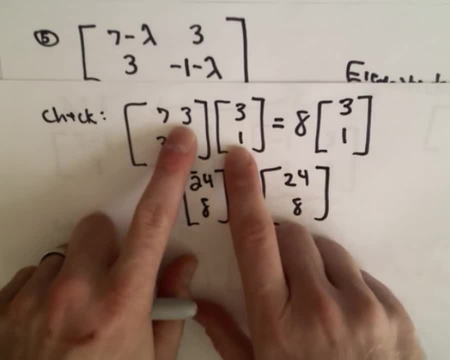 And again right. 7 times 3 is going to be 21.. 3 times 1 is 3.. So 21 plus 3 will give us 24.. 3 times 3 is 9 plus a negative 1.. 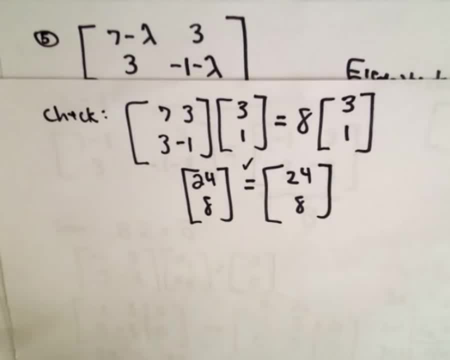 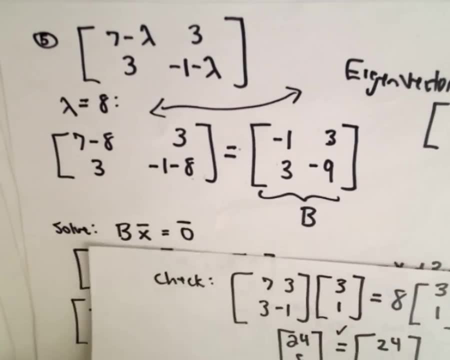 Well, that's 9 minus 1, which gives us 8 on the left. So hey, in fact that does work out. Okay, so halfway there. Now, all we have to do, we're just going to do the same process. 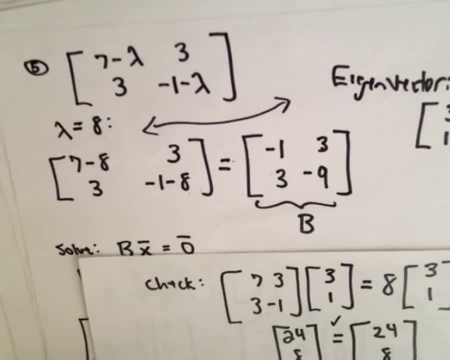 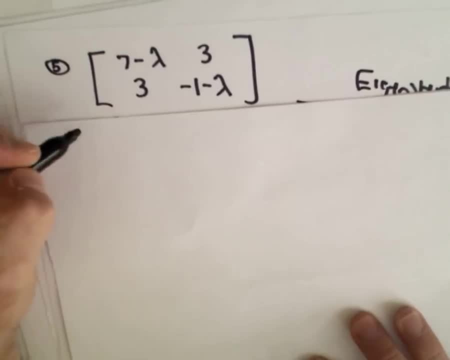 Except now I'm going to use our lambda value of what was it? I guess negative 2. And do the same thing. We're just going to do just like the exact same thing. So now, if we let lambda equal negative 2.. 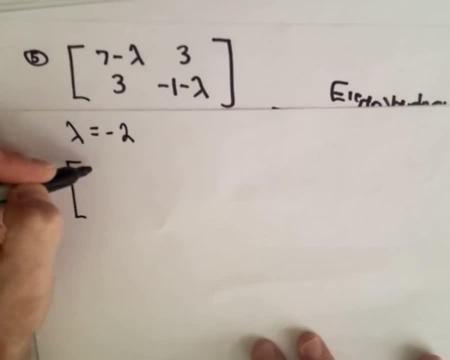 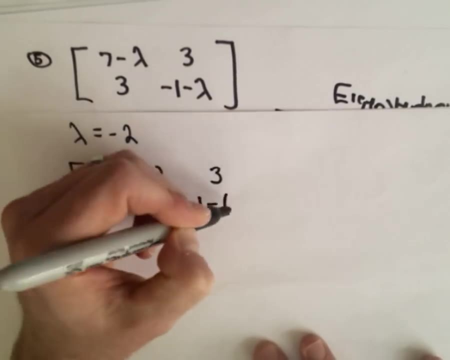 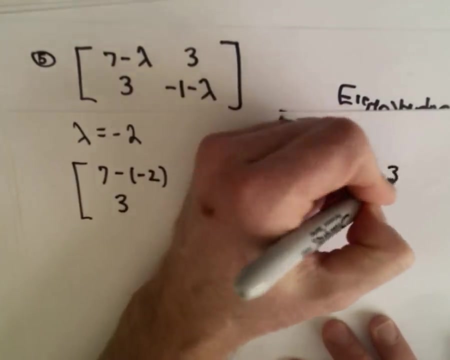 Well, in this case we're going to get we'll have 7 minus negative 2.. We've got an entry of 3.. 3, we've got negative 1 minus negative 2. And that's going to give us 9,, 3, 3.. 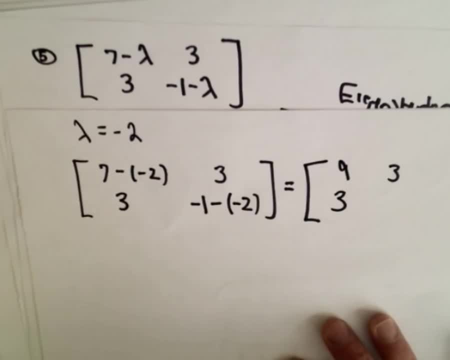 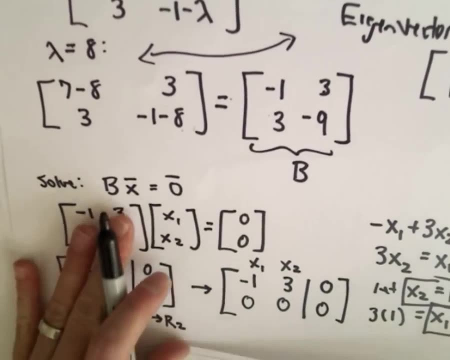 And I guess we've got negative 1 plus 2, which will give us an entry of 1.. And, just like before, what we do is we have to solve that matrix equation. So I'm just going to skip writing down this step. 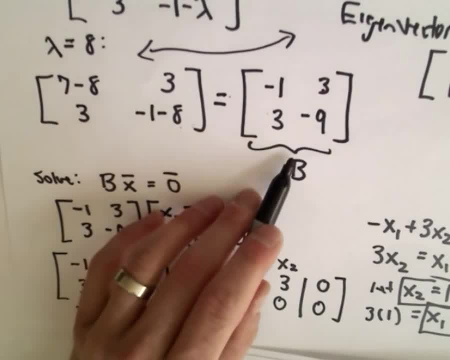 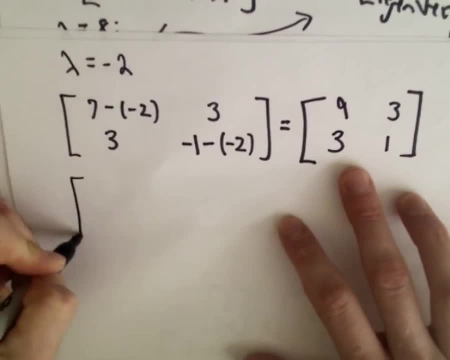 I'm just going to go ahead and jump to the row reduction, right? So once we found our matrix, we just basically did row reduction to find the relationship. So I'm going to do the same thing. I'm going to do the row reduction. 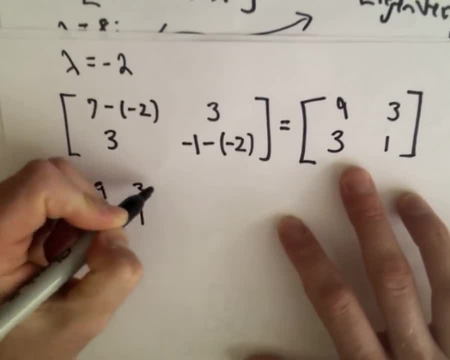 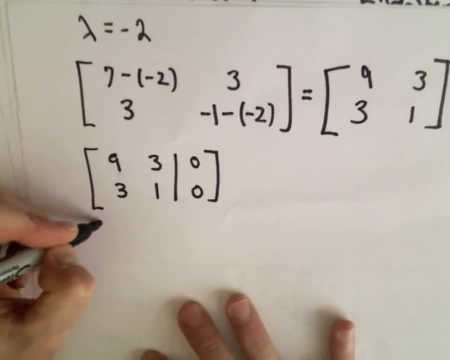 So we've got 9,, 3,, 3, and 1.. So different ways to do it. To me it looks like the most simple way is to take negative 3 times 2.. Negative 3 times row 2.. 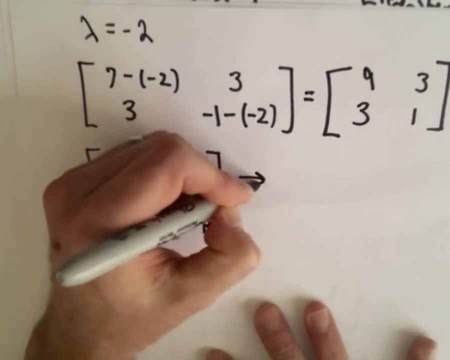 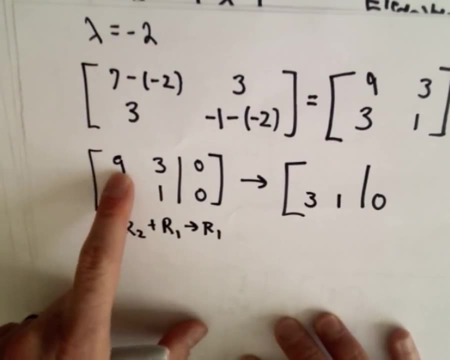 And add that to row 1 to get our new row 1.. So if we do that, row 2 is not going to change And again you can check Negative 3 times: 3 plus 9 will give us 0.. 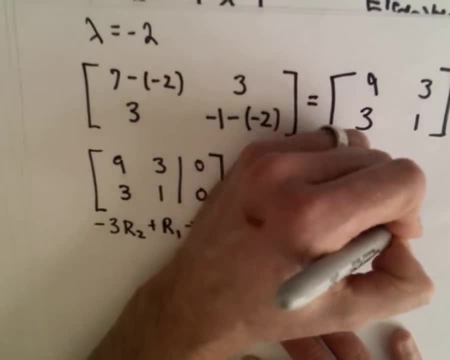 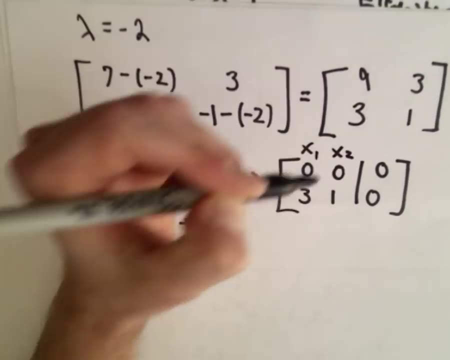 Negative 3 times 1 plus 3 will give us 0. We'll still have a 0.. 0 is at the top right And again this corresponds to x1 and x2.. So now we can write our equation. 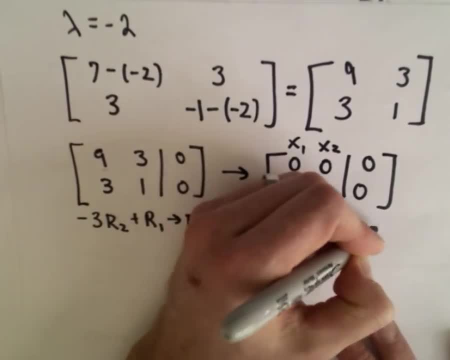 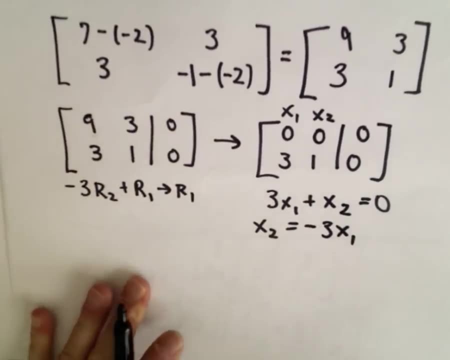 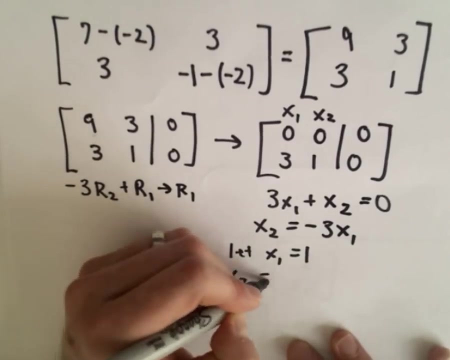 We've got 3x1 plus x2 equals 0. Or equivalently, that x2 equals negative 3 times x1.. So the same thing. You can just pick values. If we let x1 equal 1, well, in that case we'll get x2 equals negative 3 times 1 or negative 3..